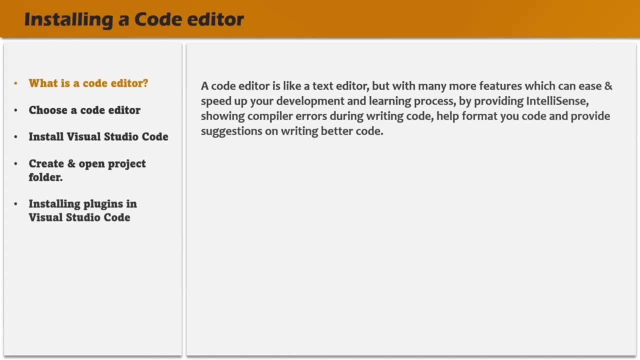 But it is not a text editor. It has many more features which can ease and speed our development process By providing intelligence, showing compiler errors during writing code, help format your code and provide suggestions on writing better code. So a code editor is like a text editor, but it is more specific for writing programs. 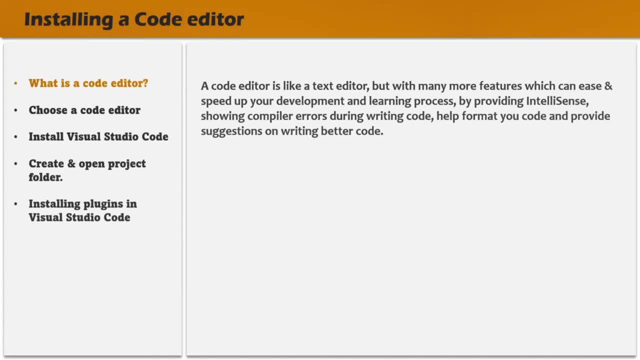 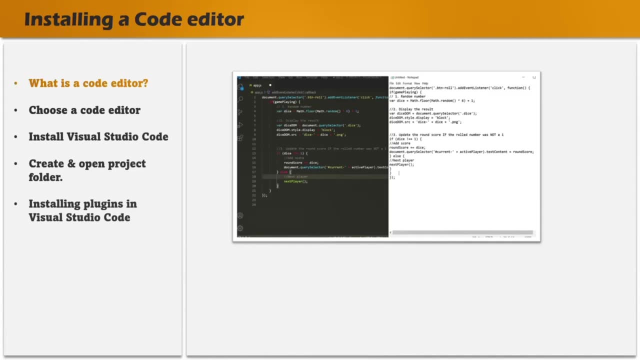 And you should always use a code editor for writing programs because it provides several benefits. So here in this image you can see that in the left hand side I have written a code in a code editor. Here I have used Visual Studio code. 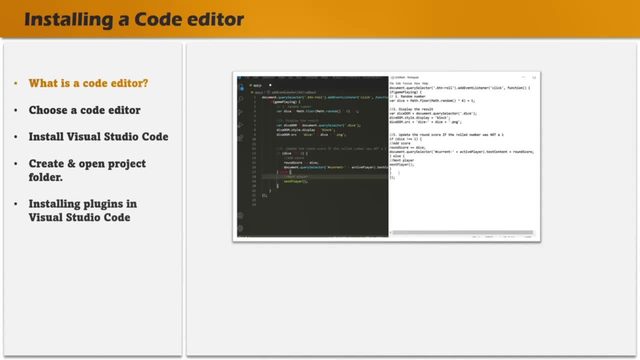 And in the right hand side you can see the same code written in Notepad, which is a text editor. Now, here you can see the program written in a code editor is more readable than the one written in the text editor. Also, code lines are properly aligned in the code editor. 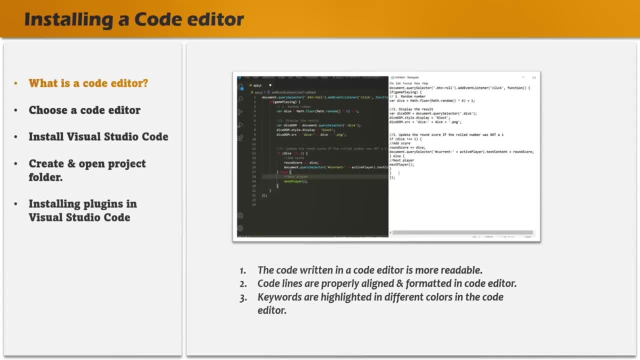 In the code editor, the keywords are highlighted in different colors, implying that these are reserved keywords, And also a code editor will display syntax errors, if any, in your program. So a code editor provides a lot of useful features which can help us speed up our development process. 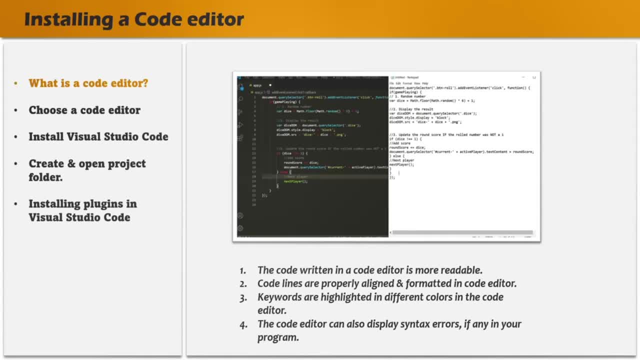 Now, if you have already installed a code editor on your machine, then you can skip this lecture, because in this lecture I'm mainly going to install a code editor on my local machine And there I'm going to install some plugins, And also in this lecture 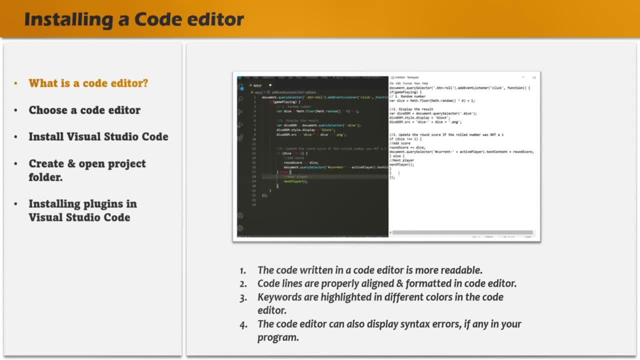 I will create a simple project where I will add an HTML file and CSS file and I will open it in the code editor. So if you already have a code editor installed in your machine, then you can skip this lecture. But if you don't already have a code editor installed on your machine, 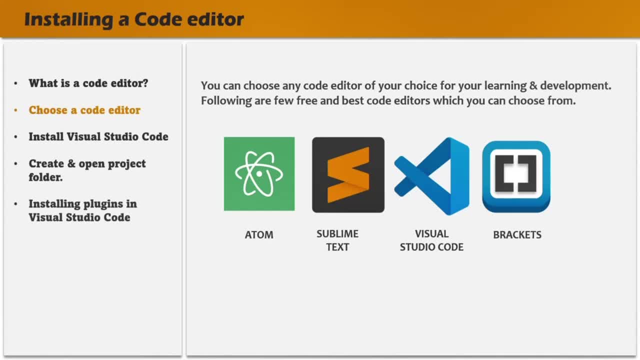 then you can choose code editor from these options. So we have Atom, we have Sublime Text, we have Visual Studio Code, we have Brackets. So all these are code editors and these are free to use. You can choose any one of them. 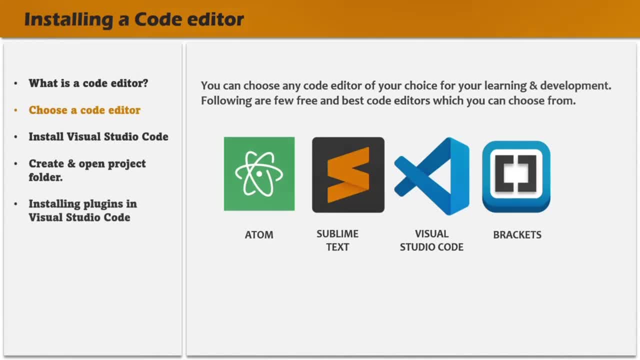 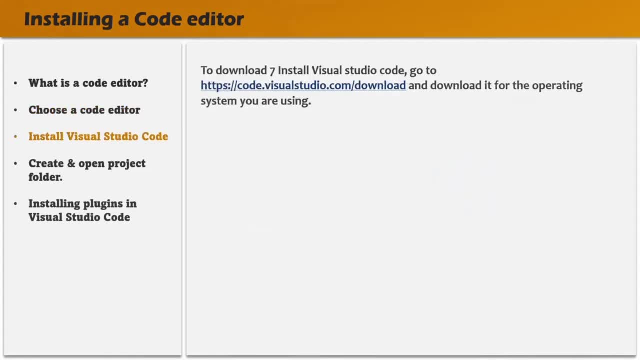 But in this course I'll be using Visual Studio Code Editor And if you want to follow along with me, you can also download and install Visual Studio Code as your code editor. Now to download and install Visual Studio Code as your code editor. 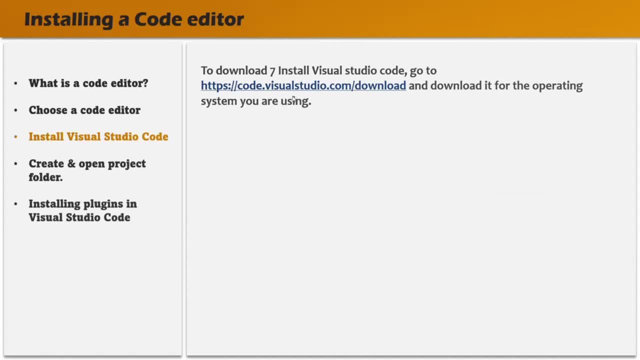 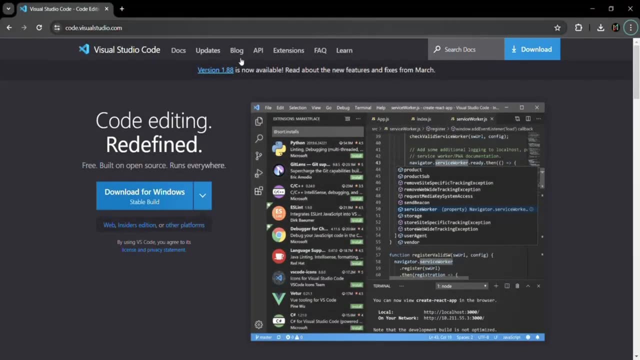 you need to go to this link. I have already opened this link in the browser, So let's go to the browser And here I have opened this link: codevisualstudiocom. Here you will see that we have this download button And here it will select the operating system of your machine automatically. 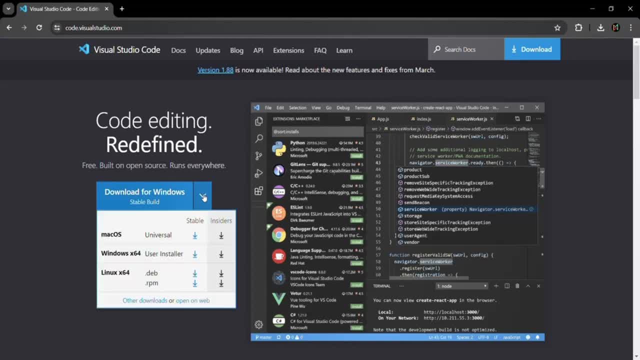 If it has not selected the operating system automatically, you can click on this dropdown and you can select your operating system. here. I'm using Windows operating system, So this option is already selected for me and I'm going to click on this download button. 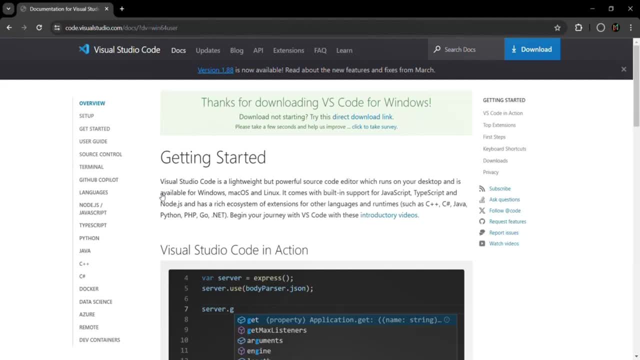 What it will do is it will start downloading the installer for Visual Studio Code, So let's wait for that download to complete. As you can see, the download is finished and Visual Studio Code installer is downloaded. Now what I need to do is I need to open this installer. 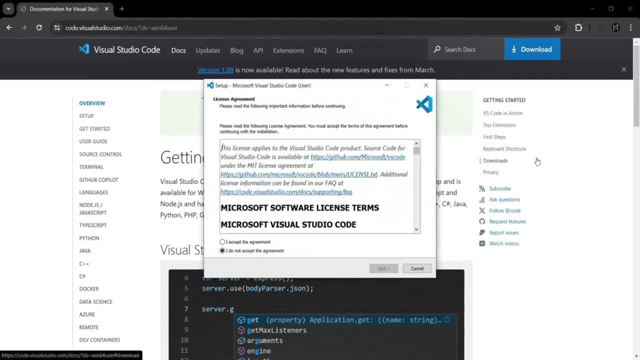 So I can simply click on that and it will open an installation window. Now here you need to accept the agreement, So click on this radio button and click on next. Then here you can select: where do you want to install this code editor? I'm going to keep the default file path here. 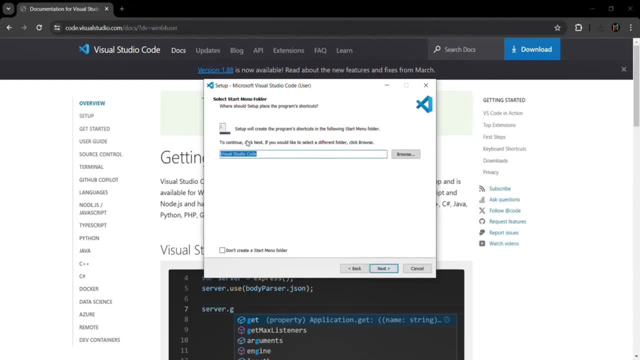 Let's click next, Then here you can see that this setup will create a program shortcut in the following start menu folder. Let's click on next here And here I'm going to keep the default settings. Let's click next again and let's click on install and it will install Visual Studio Code in my local machine. 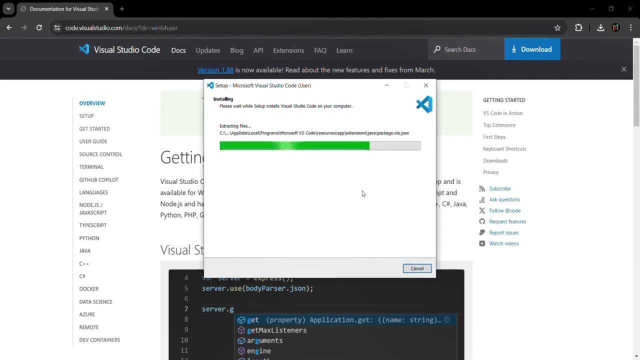 So the installation steps are very simple. You just need to follow the installation instructions and you can simply click on next on each window. Here the installation is finished. Let's click on this finish button Now. VS Code will be opened automatically here. So VS Code. 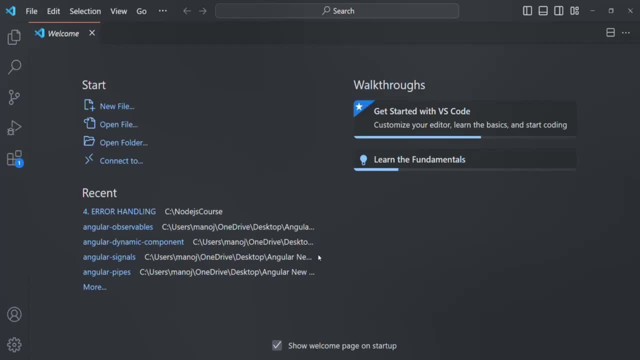 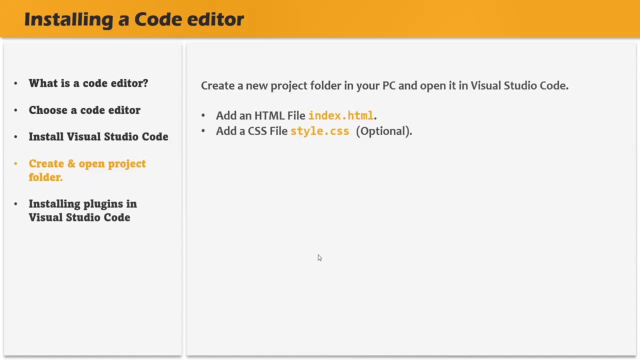 Is installed on my machine. Now, in the next step, we are going to create a new folder, a project folder, somewhere in our PC And we are going to open that folder from VS Code. For that, here I'm on my desktop. 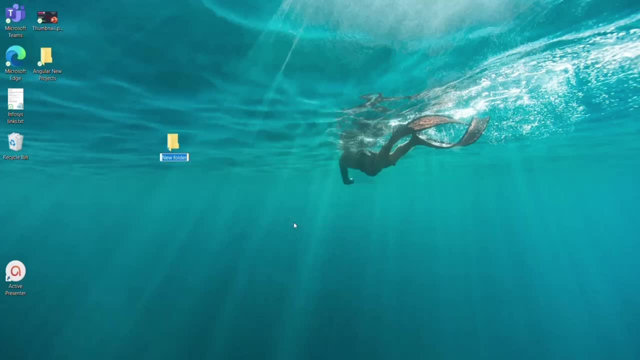 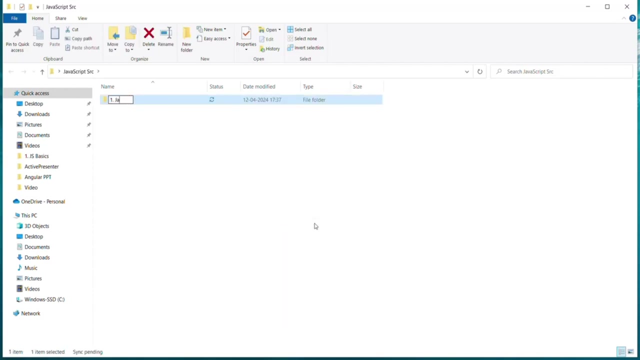 I'll right click here. Let's click on new folder And I'm going to create this folder and I'll call it JavaScript source. Okay, Inside this folder again I'll create a new folder And this one I'll call it JavaScript basics. 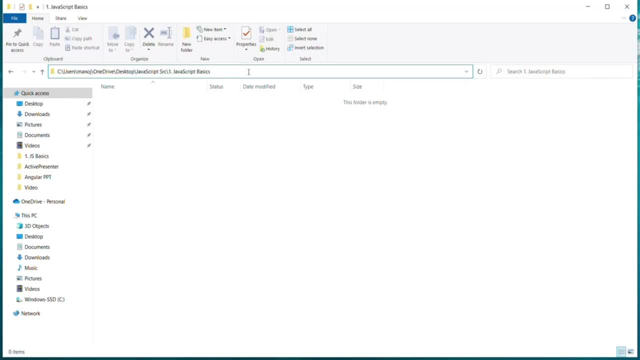 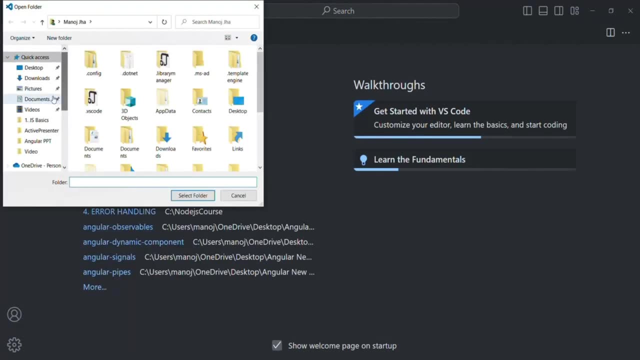 All right, Now let's go inside this folder, Let's copy the path, or maybe what we can do is we can go to VS Code itself. There we can go to file open folder. Let's go to desktop. There we have this folder: JavaScript source. 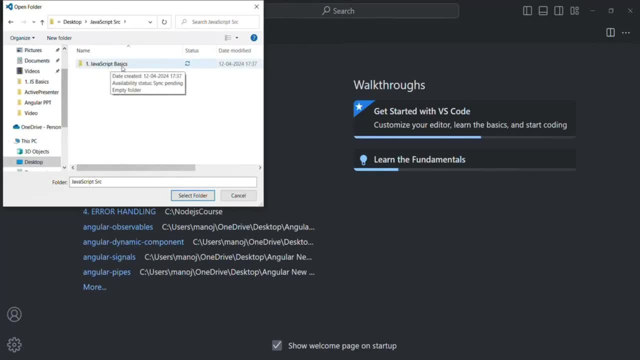 Let's go inside that And there we have this folder: JavaScript basics. So this is going to be our project folder for this section. I'll select this folder And I'll click on the select folder button. Currently in this folder we don't have any files. 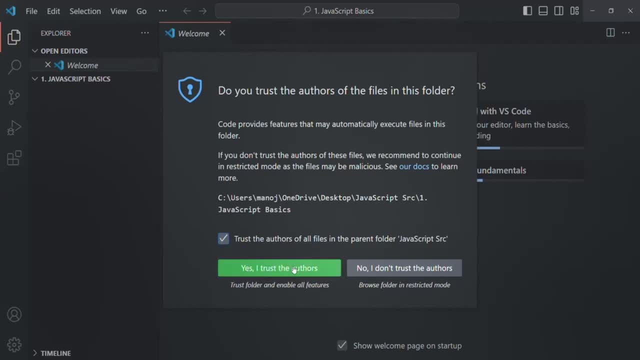 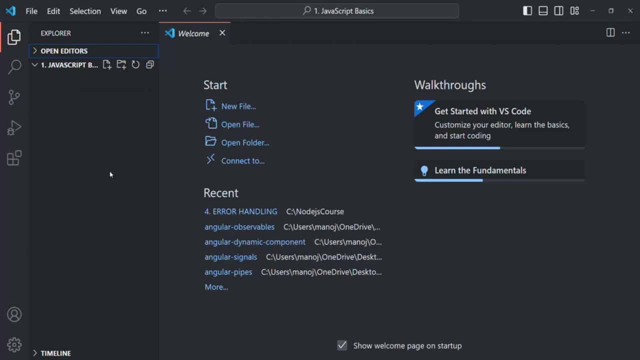 So here I can check this checkbox and I'll click on yes. I trust the authors. All right Now, currently in this folder we don't have any files, So here we are going to create two files: one HTML file and one CSS file. 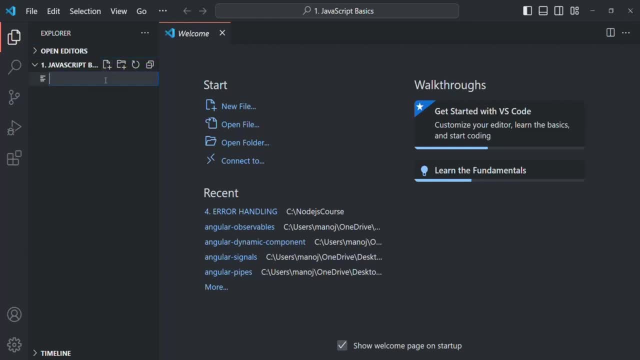 For that you can click on this button new file, And here let's provide a name, Let's call it indexhtml, Let's press enter, And that file has been created. Now we are going to write some HTML here, And for now we will simply generate a basic HTML template for that. 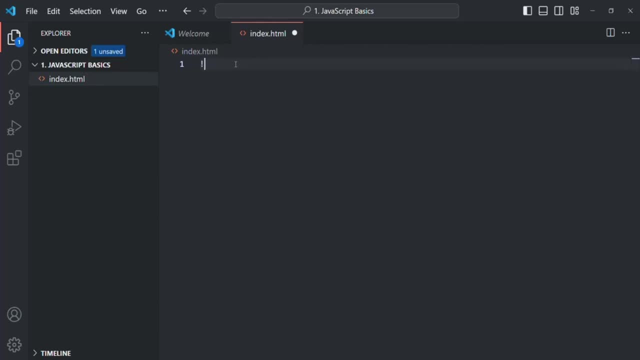 What you can do is you can press shift one on your keyboard and press tab, So it will automatically generate some template HTML for you here. If you see, in the body section we don't have anything, but it has created a basic template here. 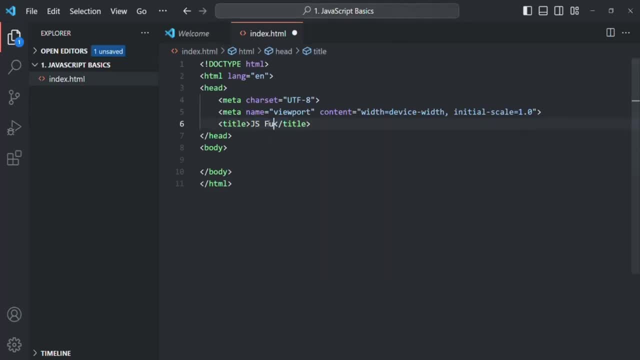 Let me provide a title- Let's say JS fundamentals, And in the body section, for now, let's simply add an H2 element and here let's say fundamentals of JavaScript. Okay, So here we have created an HTML file. Now the next thing which I'm going to do is I'm also going to create a CSS file, and I'll call it stylecss. 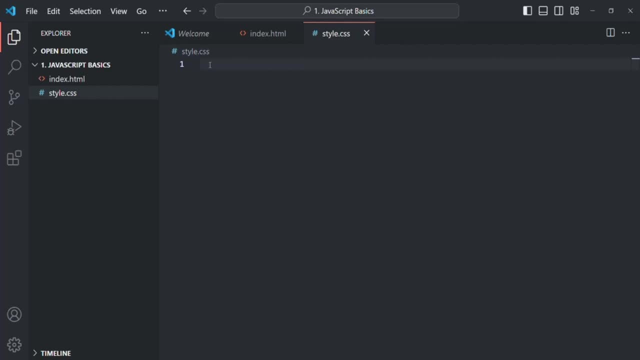 Here for now. I'm not going to write any CSS, but I'm going to link this stylecss to this indexhtml. For that let's go to indexhtml. There in the head section let's add link tag and there let's specify href to stylecss. 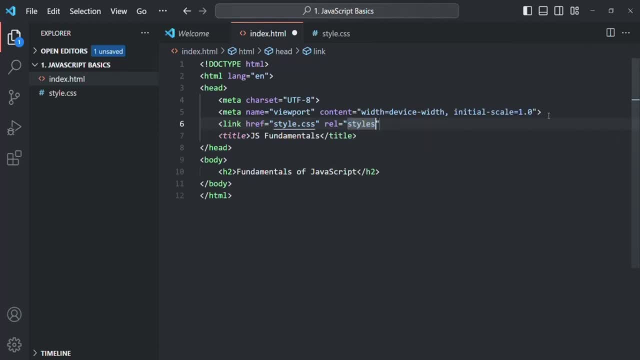 Okay, REL will be style sheet and let's specify the type as text: slash CSS. All right, Let's save the changes And, just to test it, what we will do is here for the H2 element, Let's add a simple style. 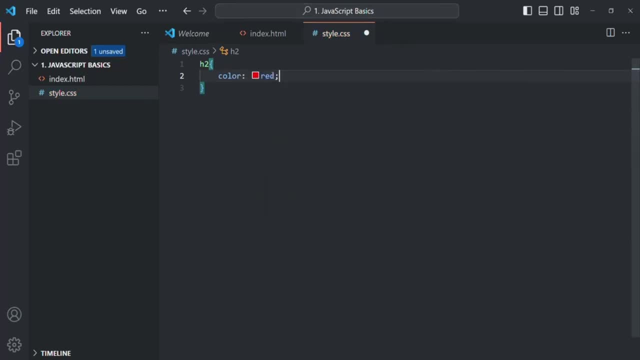 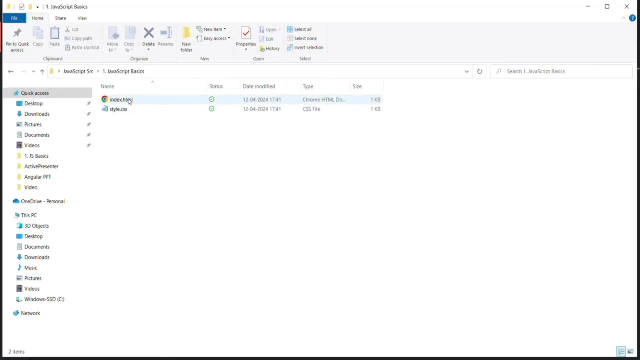 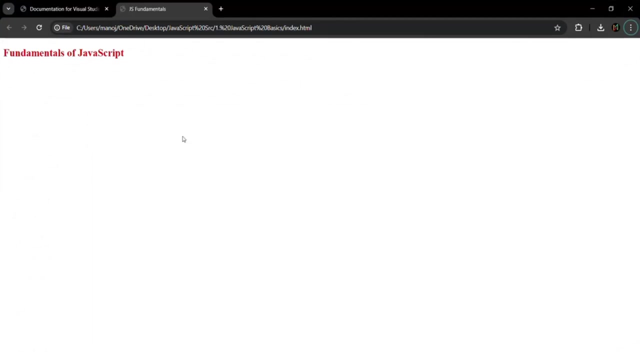 Let's set the color to maybe red, Let's save the changes. Now let's go to our project folder and there let's double click on this indexhtml to run it in the browser, And now you can see the HTML which we have written in indexhtml. that has been rendered here. 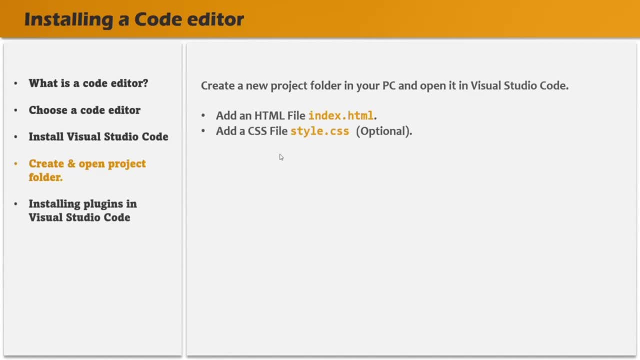 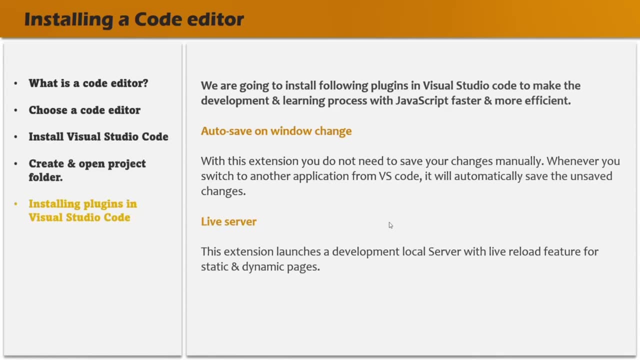 All right. Now what we are also going to do is we are going to set the color. So what we are going to do is we are going to install some plugins for our Visual Studio code, And we are going to install two plugins: autosave on window change and live server plugin. 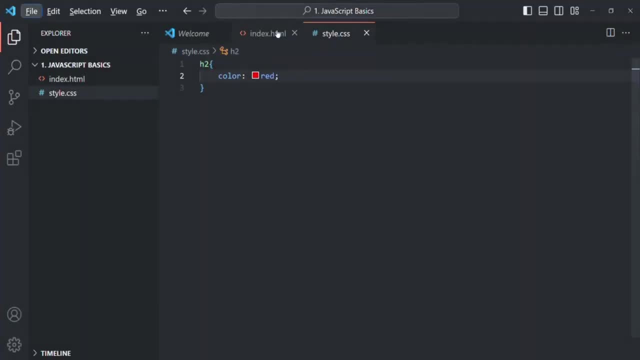 So currently what is happening is if I go to indexhtml and if I do some changes here, if I don't save it and if I go to the browser, you will not see that change. For that you will have to first save it. 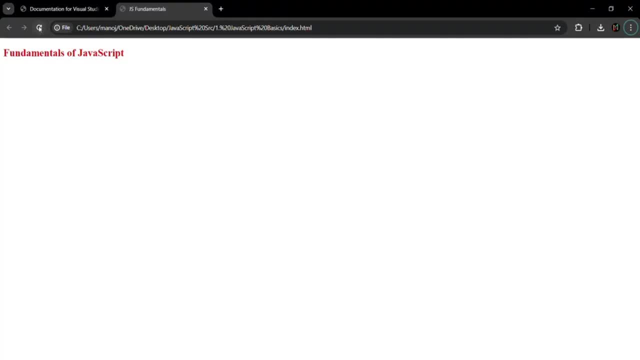 And then now, when you go to the browser, you will not see that change. So when you go to the browser and when you refresh the page it will show that change. So currently we have to manually save our files. 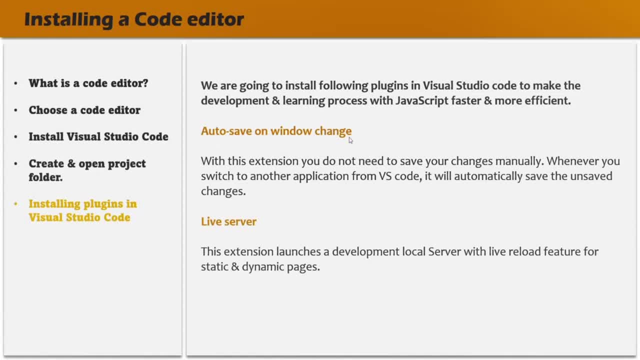 But using this plugin, autosave on window change. what it will do is whenever the window will change. whenever we move from Visual Studio code to some other window, the changes will be saved automatically. So we will not have to manually save our changes every time we change something in the file. 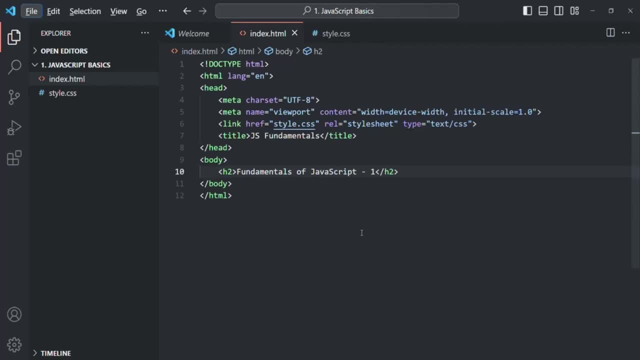 So let's go to VS Code To install a plugin. you need to go to this extensions section here. There you will see a lot of extensions, a lot of plugins which you can add for your Visual Studio code. But here let's search for autosave on windows change. 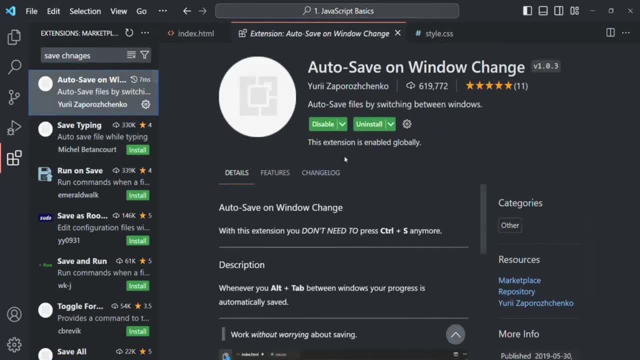 Okay, so this is a plugin name. Let's click on that, And currently it is already installed for me. But if it is not installed for you, you will see the install option here. You can simply click on that and it will install that plugin for Visual Studio code. 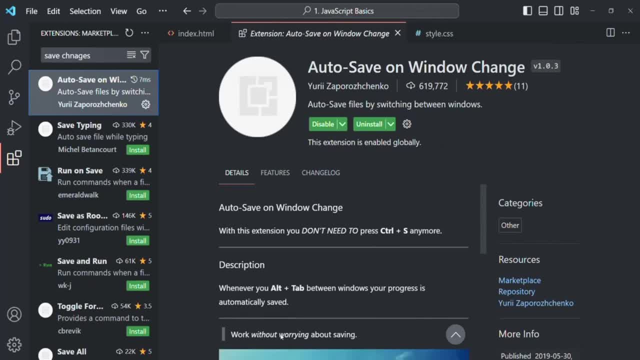 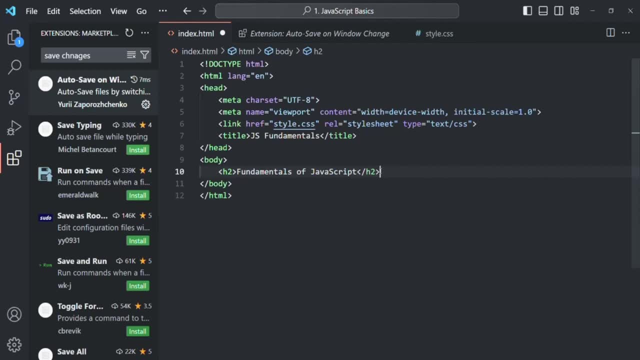 Okay, so now, every time we will make some changes in our file, it will be automatically saved. If I remove it from here. currently this file is not saved. That's why you will see this white dot here. But as soon as I change the window, as soon as I move away from Visual Studio code. 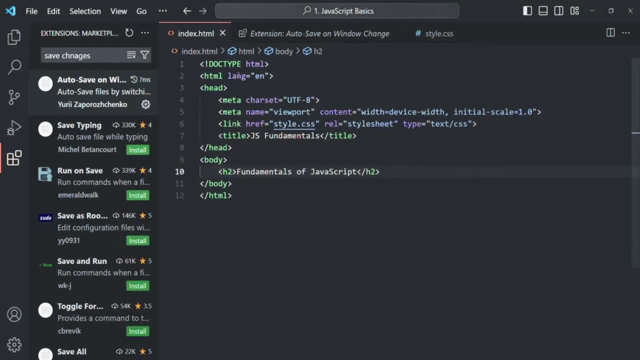 let's say, if I go to the browser and if I come back again, you will see that it has automatically saved. So this is the use of this plugin: autosave on windows changes. Now the next plugin which we want to install is this live server plugin. 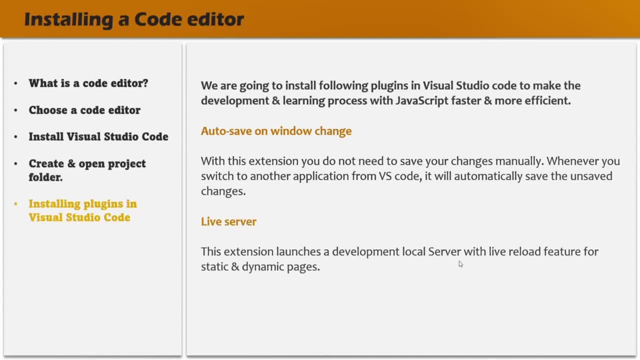 And what this plugin will do is. it will launch a live development server in our local machine and it will run our indexhtml file in that live development server. Currently, what we did is we double clicked on this indexhtml file and it opened it in the browser. 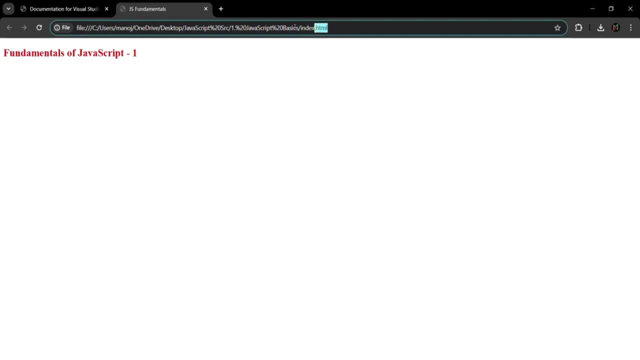 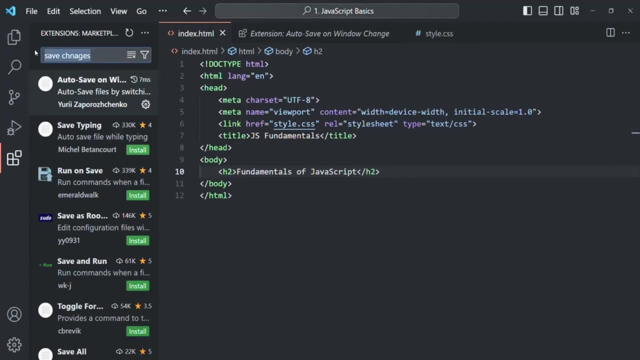 But here in the URL bar you will see that it is showing the path of that file, The complete path of that. But I want to run this indexhtml file in live development server. For that let's go back to VS Code and here let's search for live server extension. 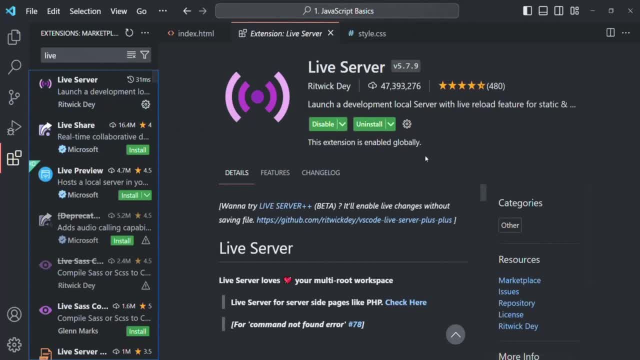 So here we have this live server extension. Click on that and again it is already installed for me, But if it is not installed for you, you will see an install option here instead of uninstall. Again, you can click on that button and it will install this extension, this plugin for Visual Studio code. 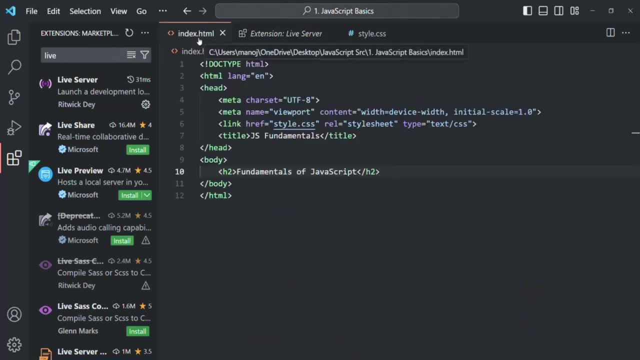 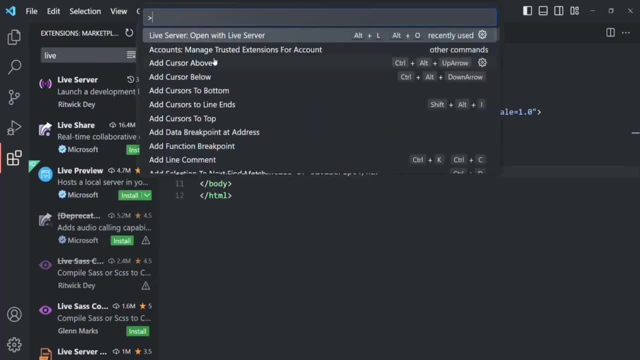 And now, if I go to indexhtml there, if I go to view command palette, there you can search for live server. It is already showing me here. So when I will click on this option, what it will do is it will open this indexhtml file in a live development server. 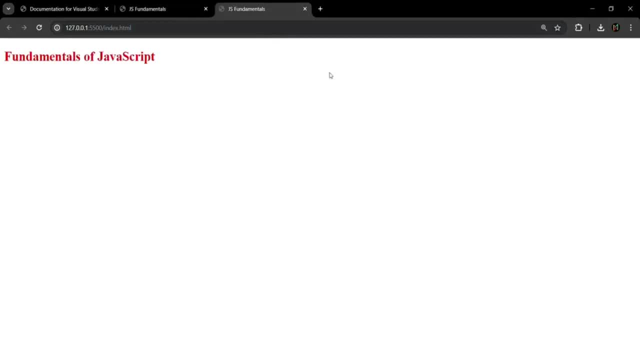 So if I click on it you see it has opened it in a live development server And here in the address bar you can see that this indexhtml file, Our application. it is running on this IP address, 127.0.0.1,, which is the IP address for local host. 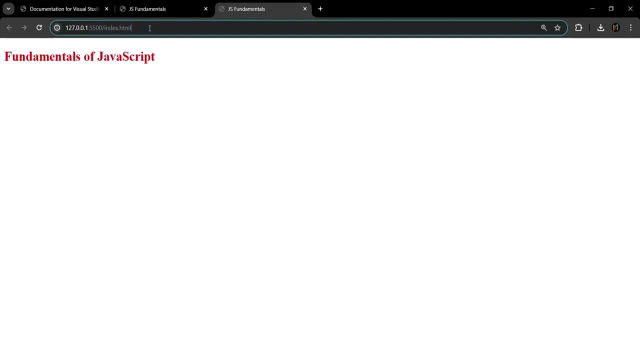 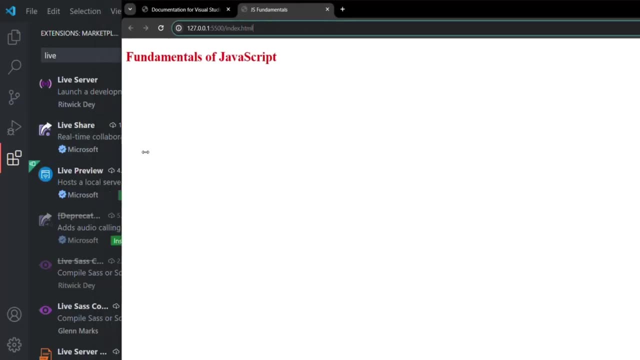 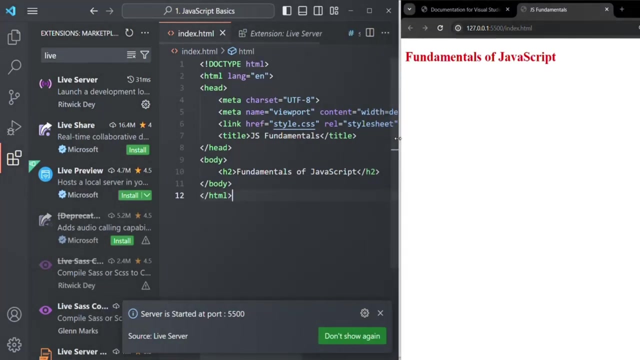 And it is running on port number 5500.. Okay, So let me close this one and let me also resize this window here, Like this, And let's also resize this window. Okay, Okay Now, If I do some changes here.